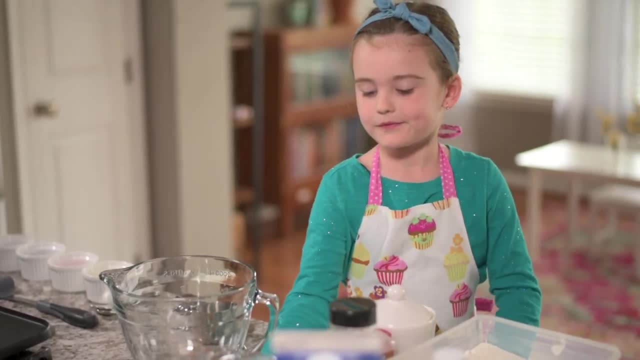 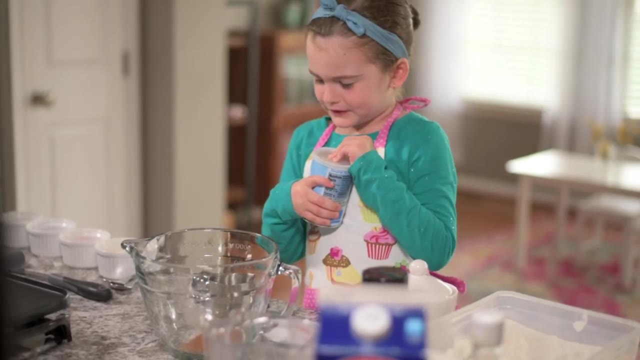 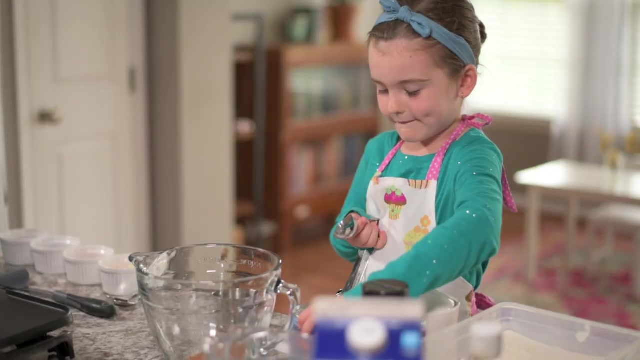 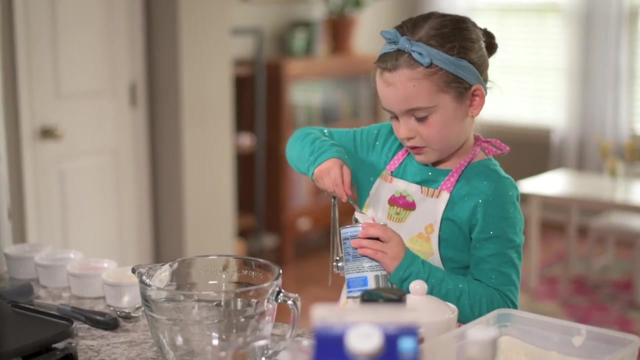 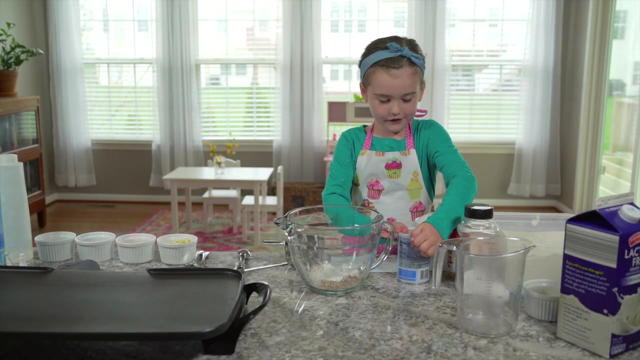 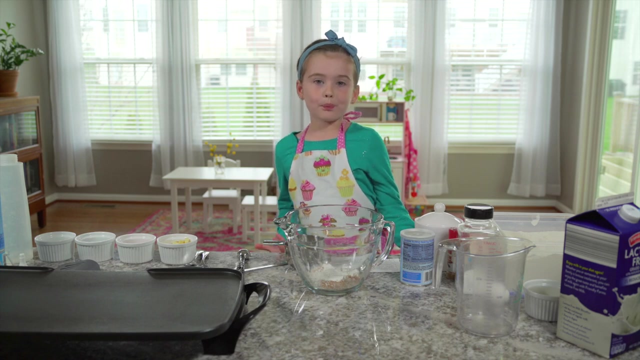 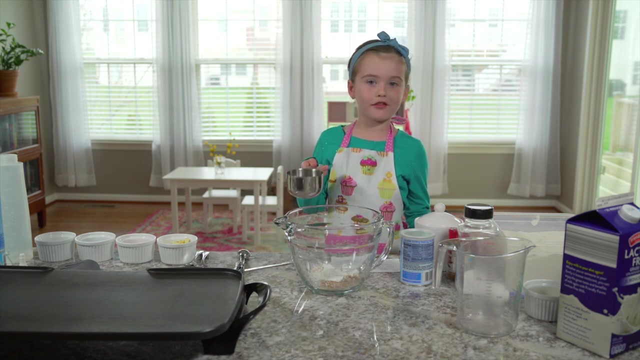 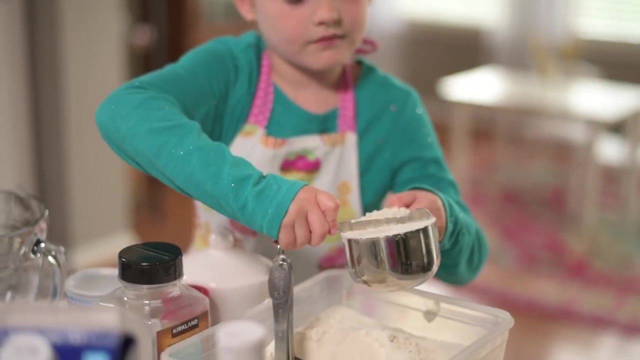 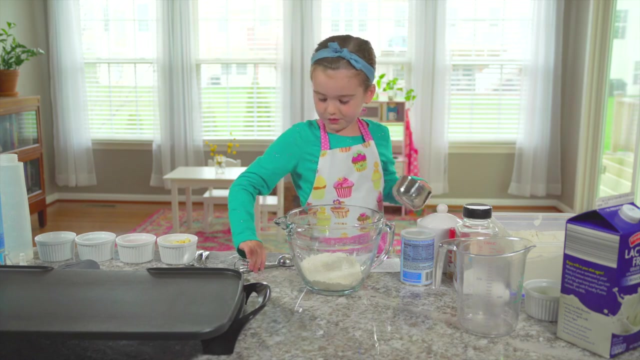 After that you use a little bit of baking powder- One tablespoon of baking powder. After you have put the baking powder in your bowl, then you have to add one cup of flour. If you measure it well, then it will be the size you want and 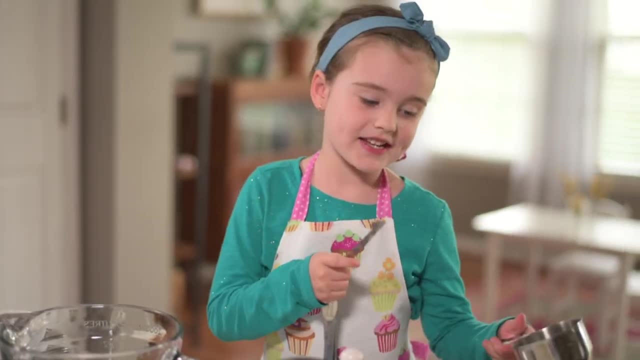 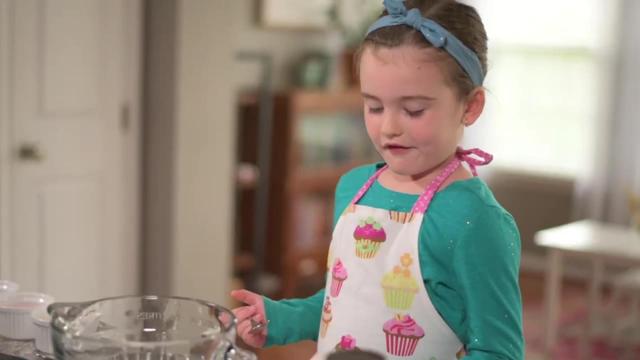 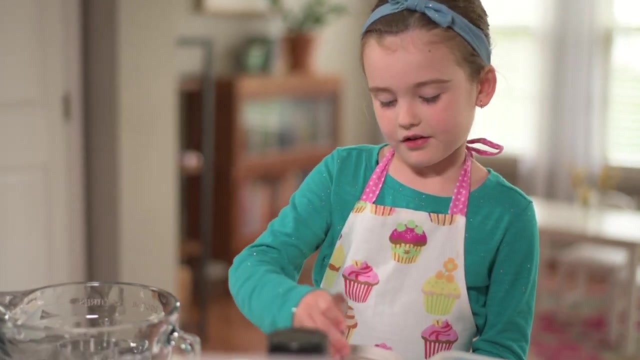 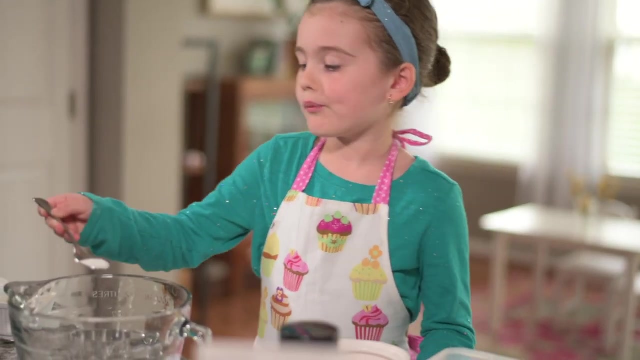 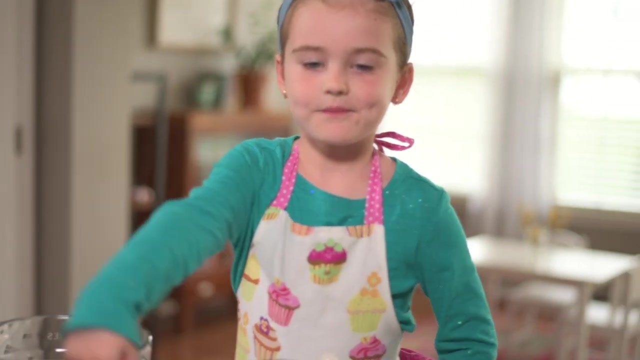 it will taste as good as you want it to. Then, after you have put your flour in the bowl, you have to add a spoon of sugar. I like to do a half too. Now it's time for the wet ingredients. You have to add one cup of milk. 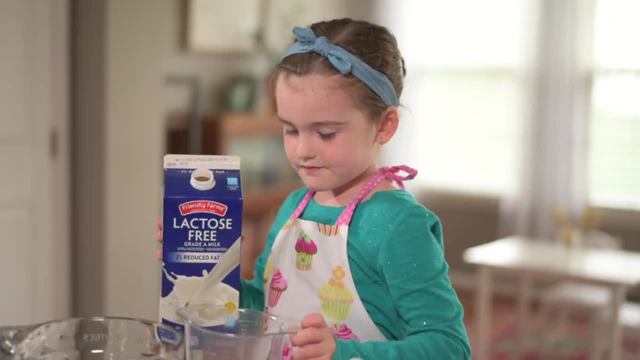 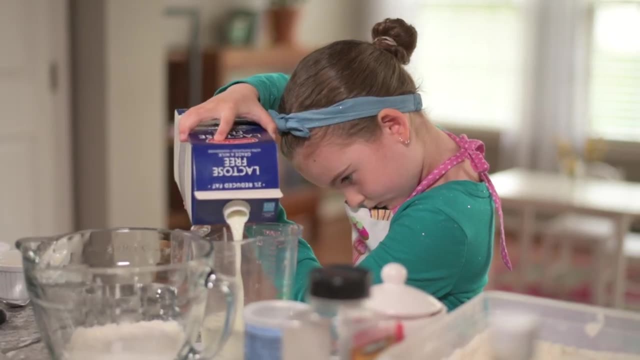 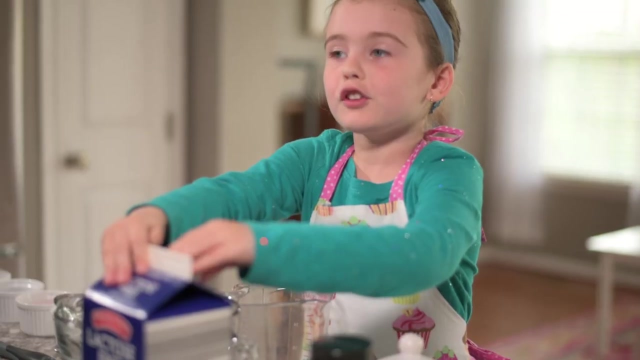 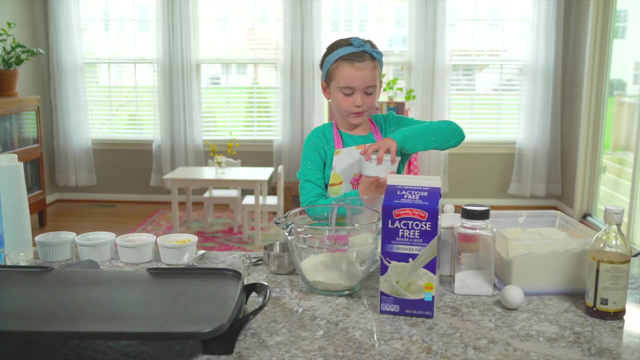 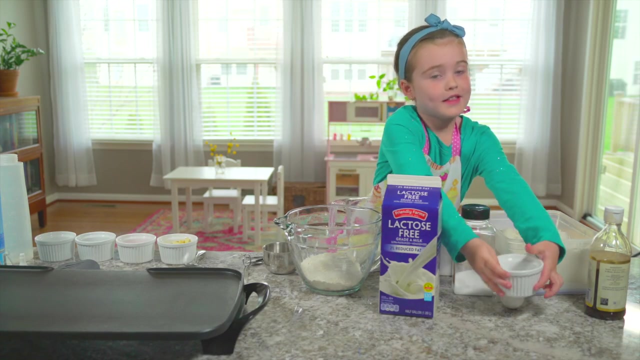 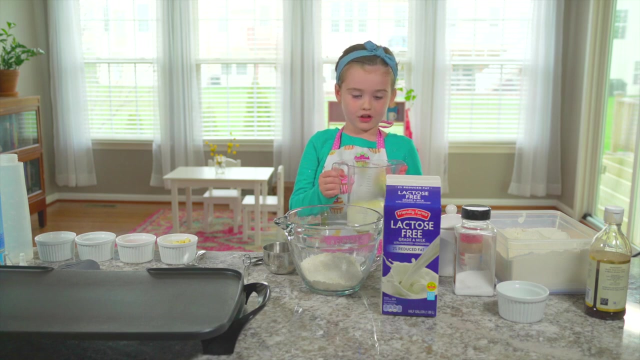 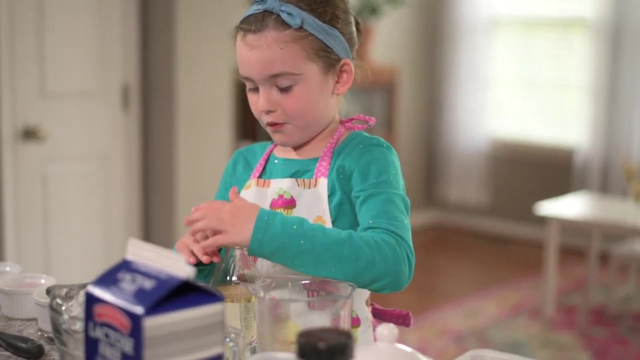 After you put the milk in, you will need vegetable oil. You have to add one cup of milk. After you have put the vegetable oil in the measuring cup, then you will need to add a little bit of vanilla That exploded. That's good. 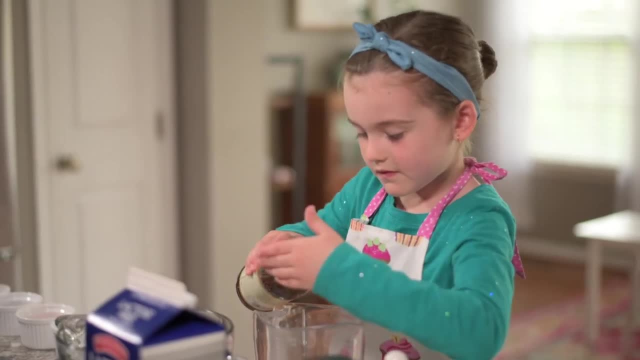 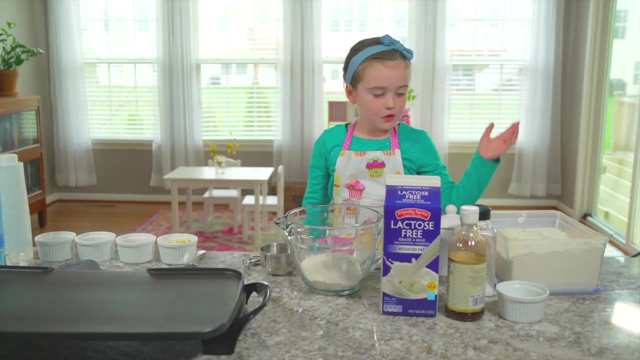 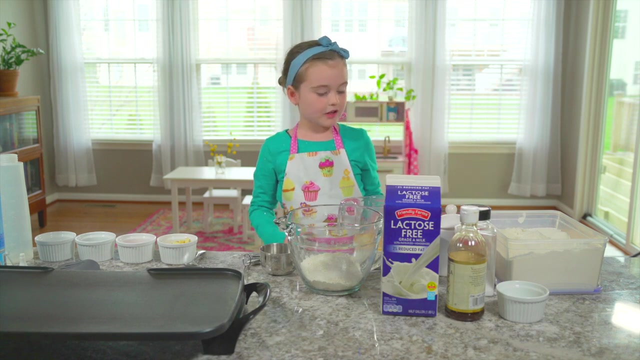 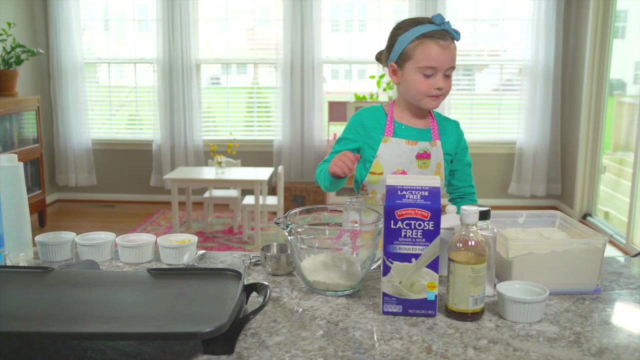 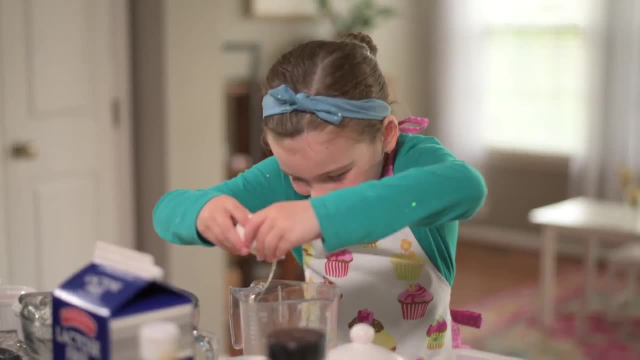 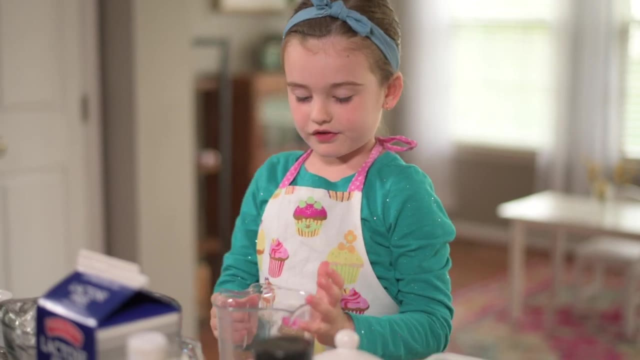 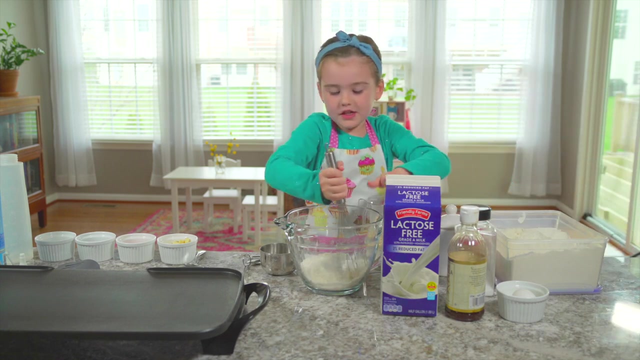 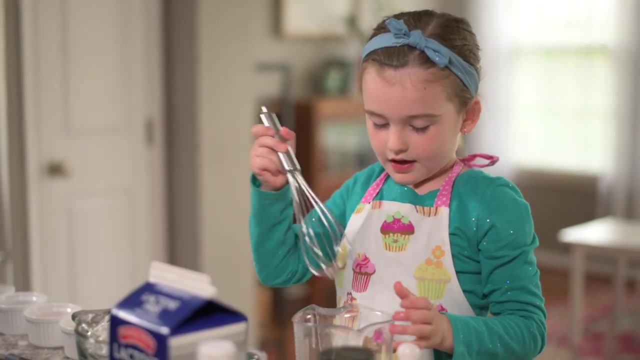 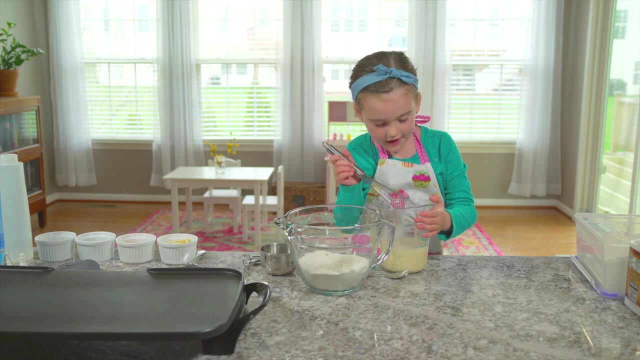 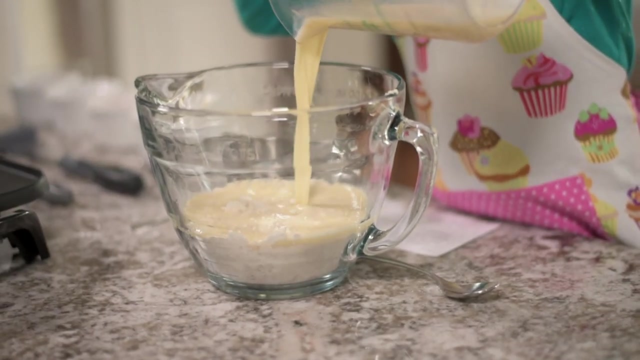 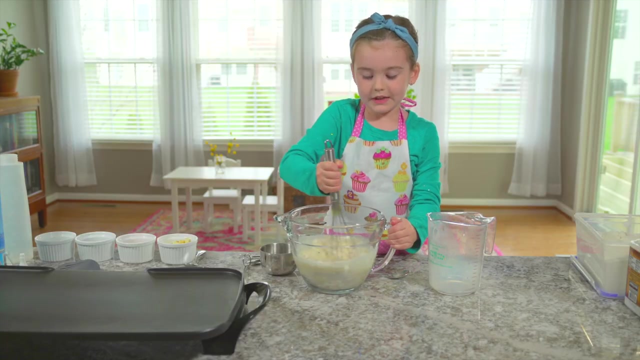 Whoa. If you have done all of the wet ingredients, then it is time to whisk the dry ingredients together And then, after the wet ingredients, After that is done, you will have to pour the wet ingredients into the dry ingredients. Then you will have to mix it. 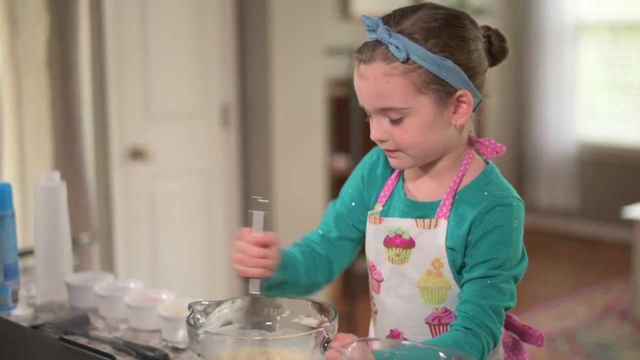 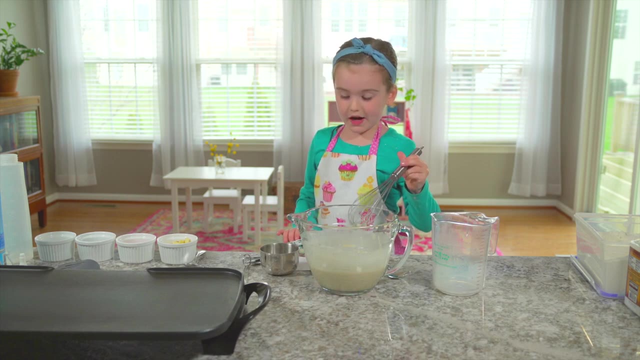 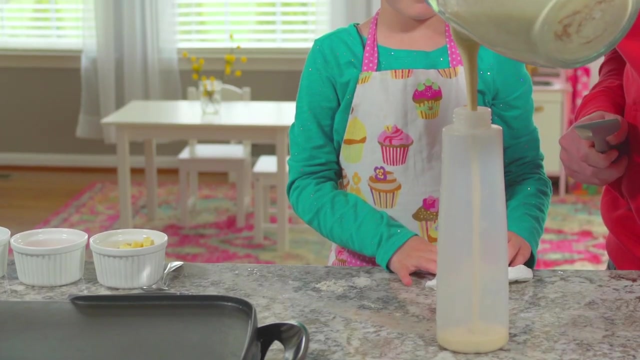 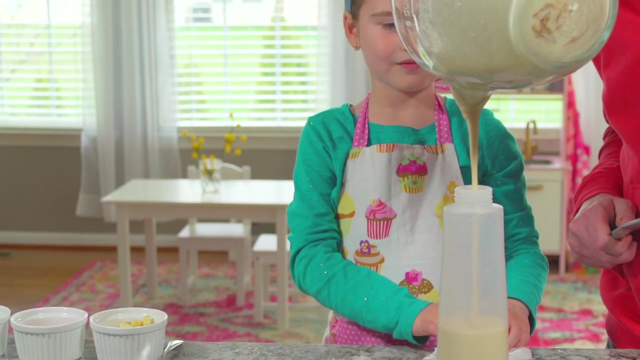 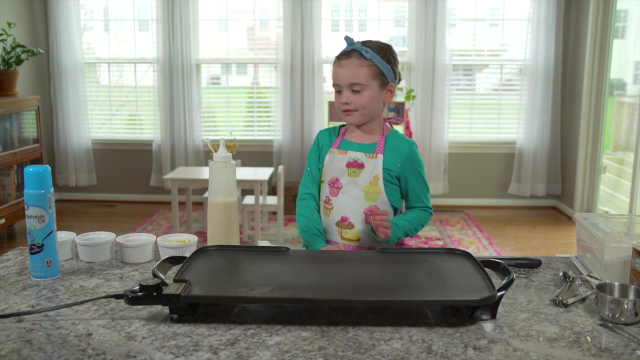 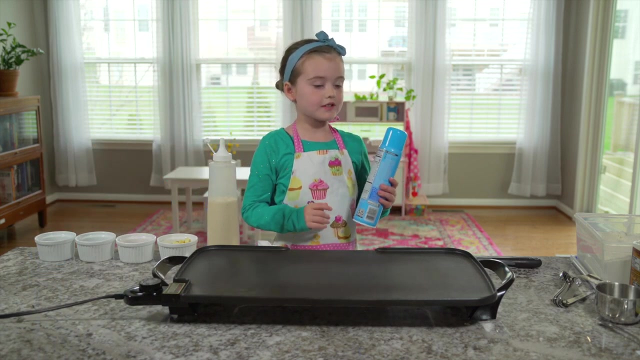 Okay, And you might need some help from your parents, because this is when it gets a little bit messy. After you have done this, After you have done that, you have to grease the pan or the griddle, And I'm going to show you how to do that. 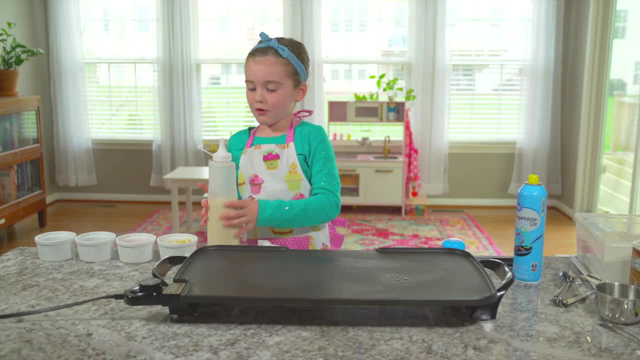 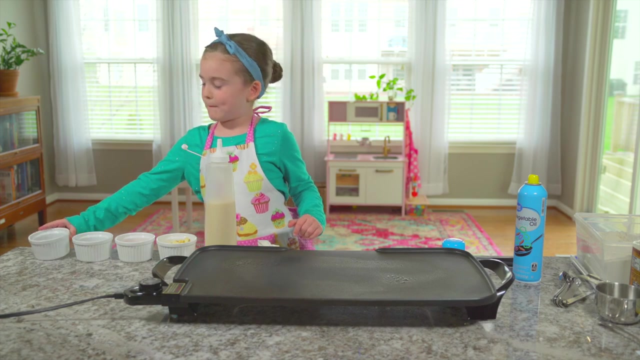 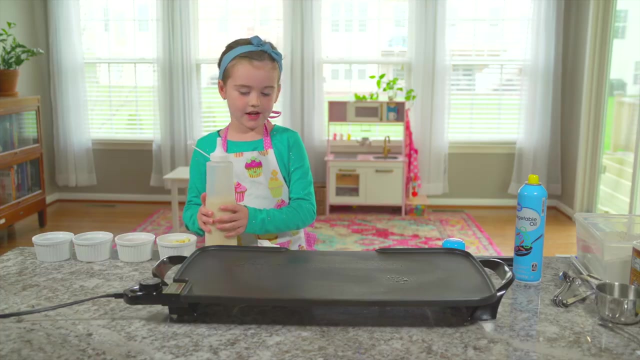 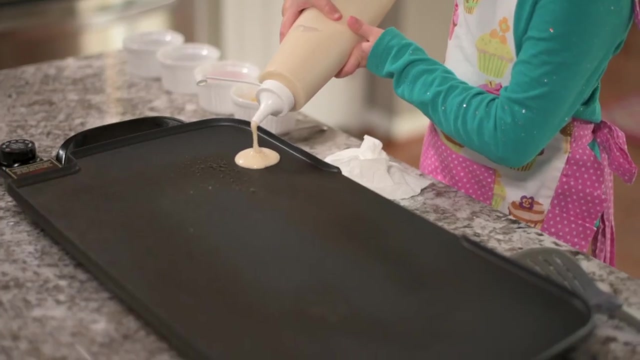 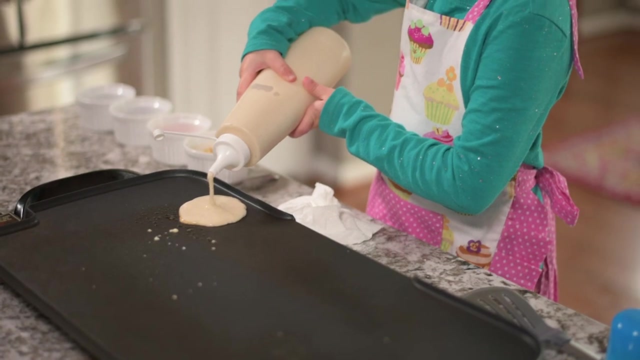 I'm going to make four different kinds of pancakes: Banana, strawberry, blueberry and chocolate chip pancakes. So now I am going to make the pancakes. Okay, Add 1 teaspoon of salt and 1 teaspoon of black pepper and mix well. 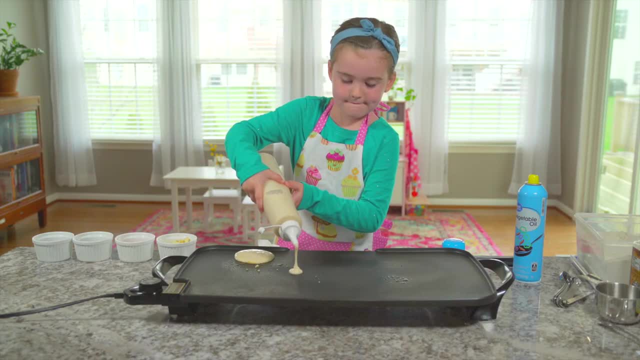 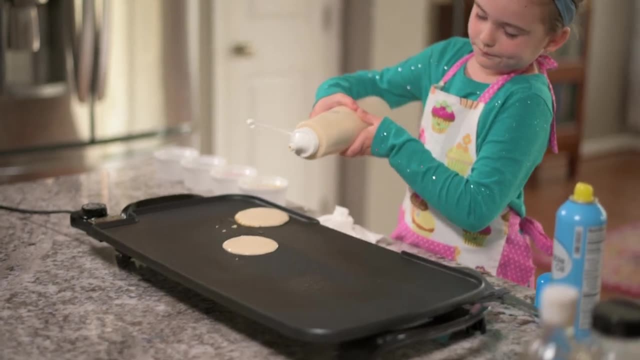 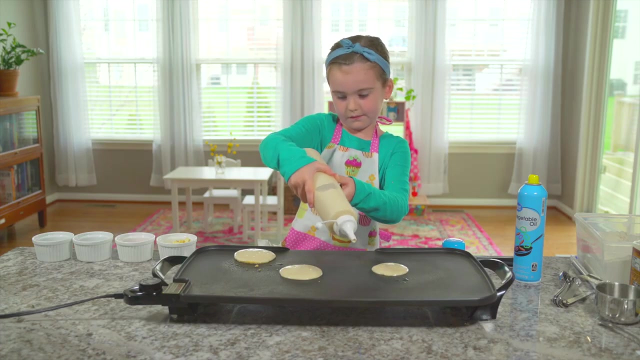 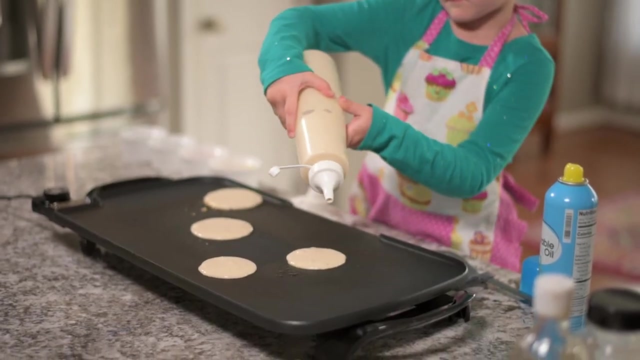 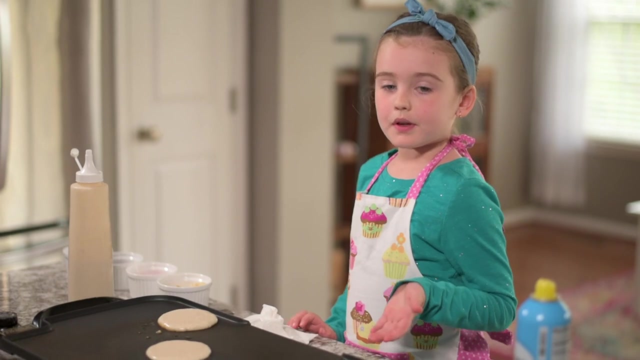 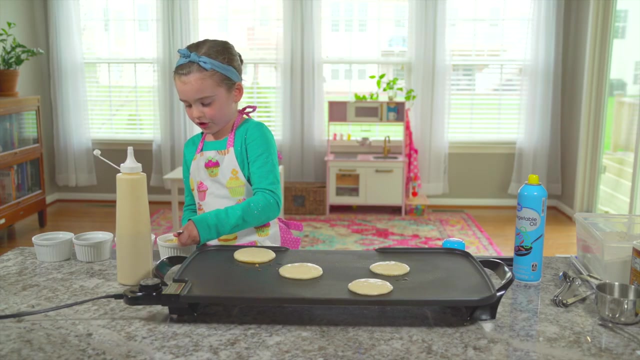 Add 1 teaspoon of black pepper and mix well. Add 1 teaspoon of black pepper and mix well. Add 1 teaspoon of black pepper and mix well. After you have put the pancake onto the griddle or stove, you can add the toppings. 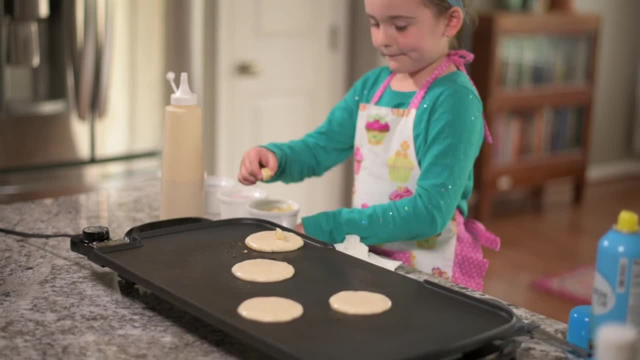 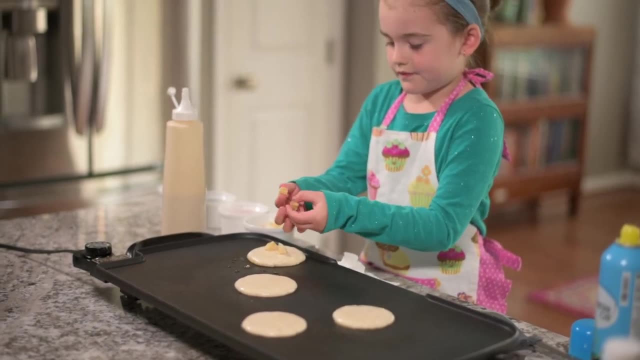 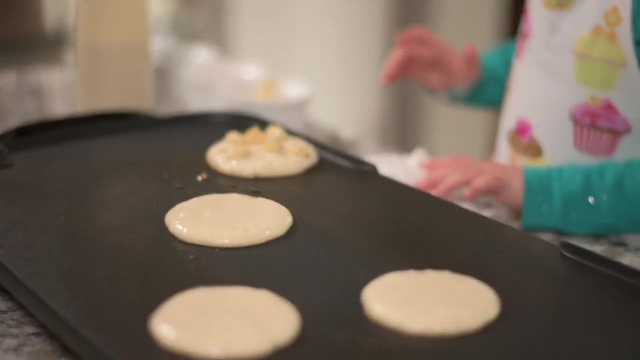 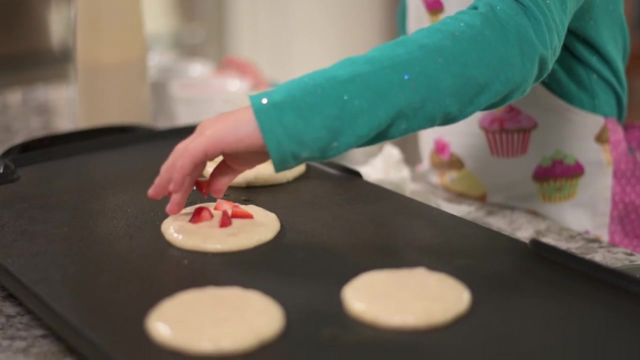 After you have put the pancake onto the griddle or stove, you can add the toppings. After you have put the pancake onto the griddle or stove, you can add the toppings. You can also use a spoon for this. Now I'm going to add the strawberries. 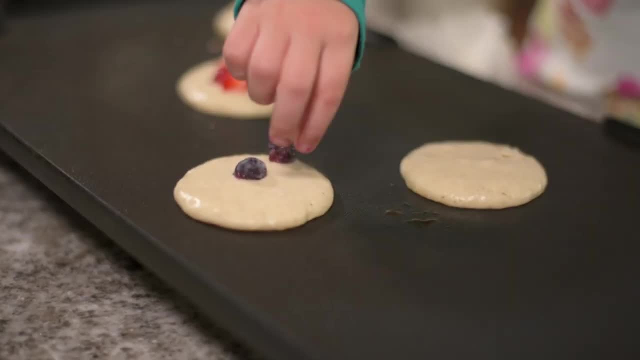 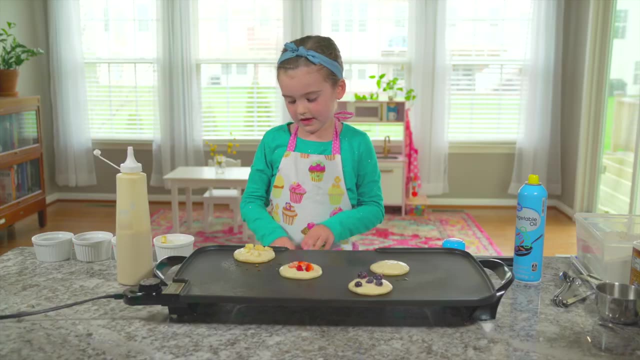 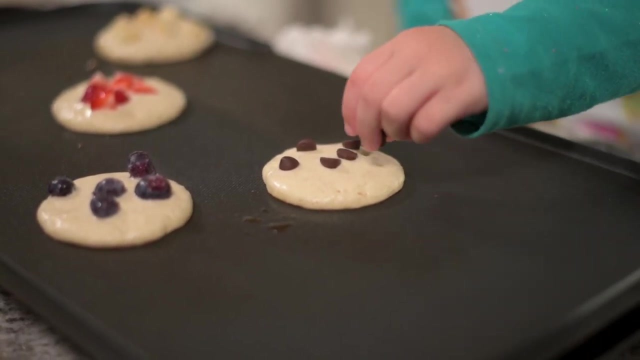 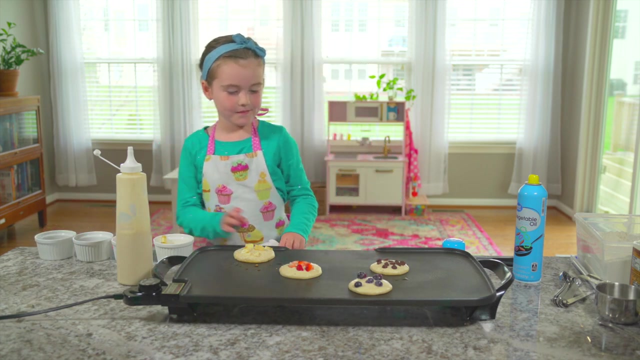 It kind of looks like a star. After you can do the rest, like blueberries: Now I'm going to do chocolate chips. Now I'm going to do chocolate chips. Now I'm going to do chocolate chips. This one has a lot. 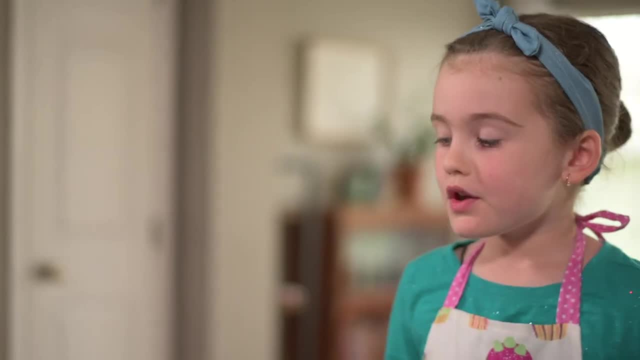 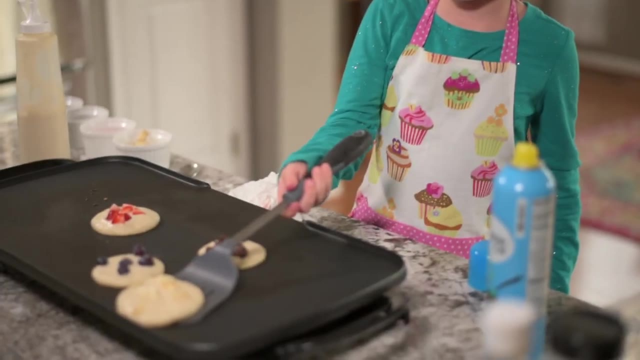 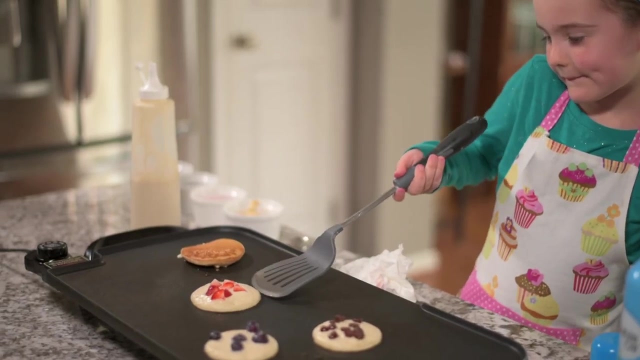 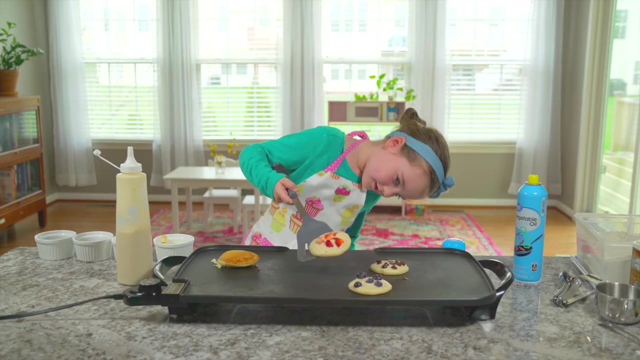 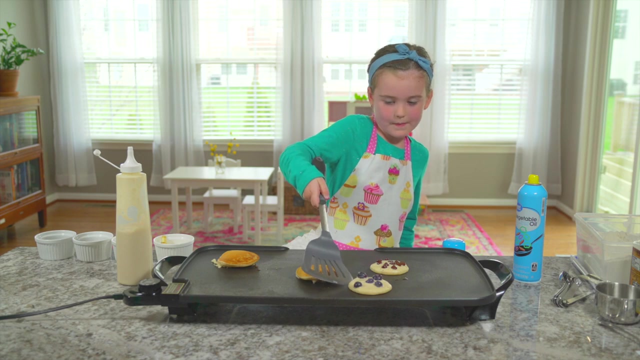 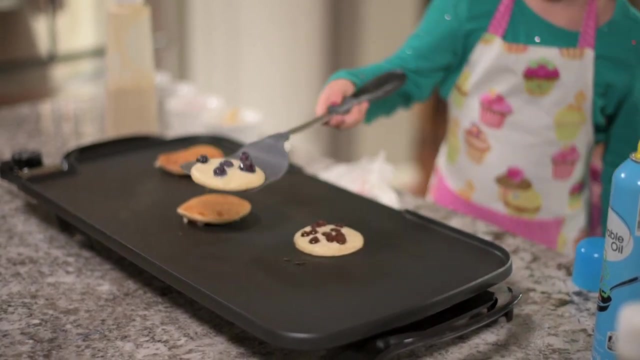 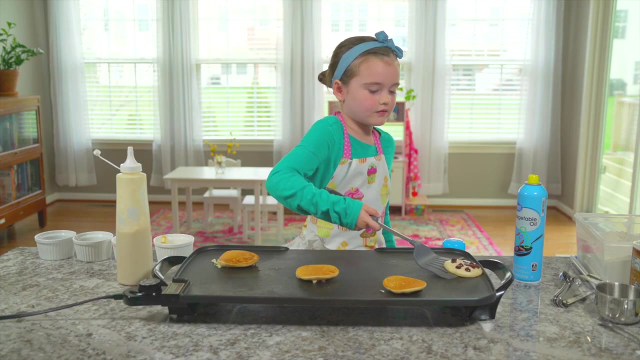 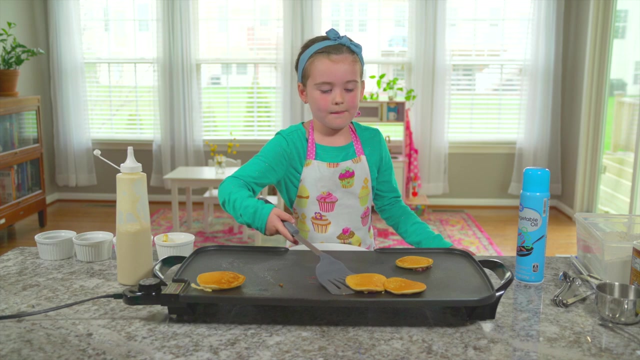 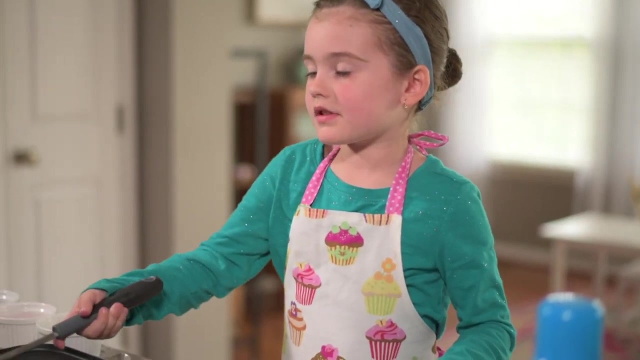 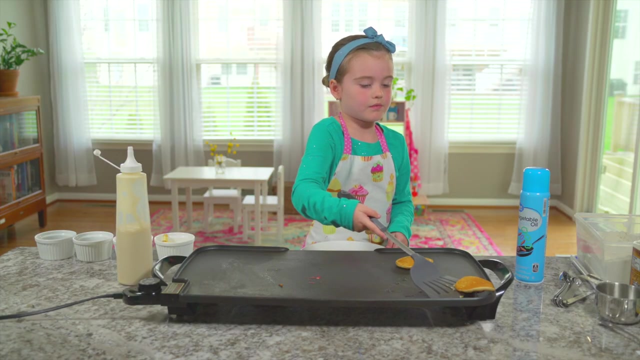 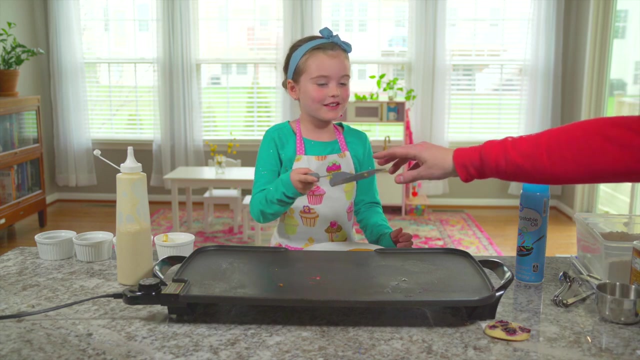 After you wait a minute or two, you can flip them. Let's check. Sometimes you have to chase it, I don't know, And maybe sometimes you don't really need to. Oh no, That was weird. Maybe sometimes there's a little mistake, but that's okay.